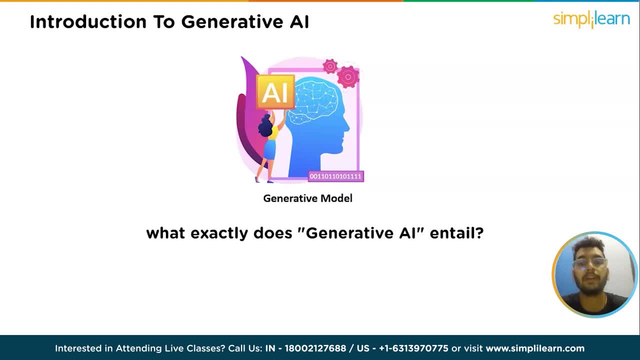 better understanding of how this technology operates and its growing integration to our daily lives. Generative AI is, after all, a tool that is based on artificial intelligence. A professional who elicits to switch careers with AI by learning from the experts, Then try giving a short. 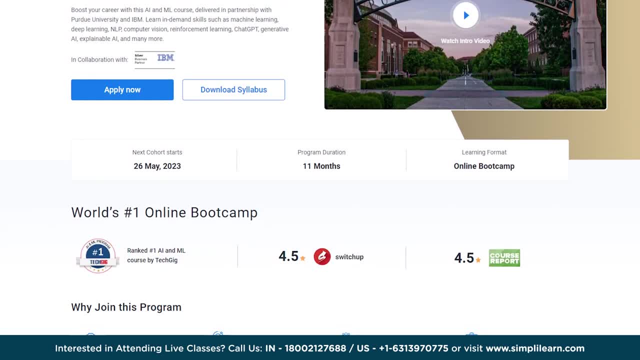 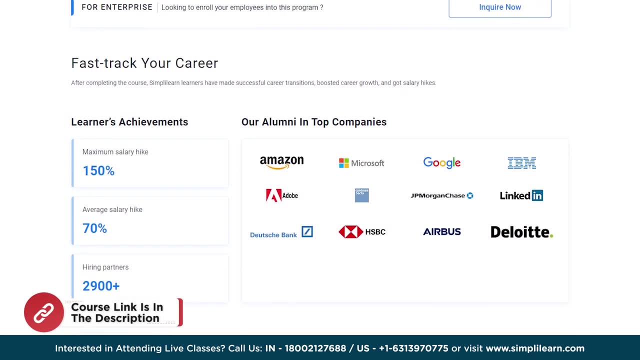 simple postgraduate program in AI and machine learning from Purdue University in collaboration with IBM. The link in the description box should navigate to the home page, where you can find a complete overview of the program being offered. Take action, upskill and get ahead. 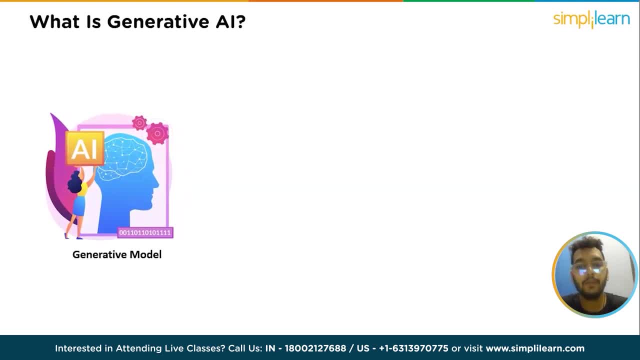 What is Generative AI? Generative AI is a form of artificial intelligence possessing the capability to generate a wide range of content, including text, visual, audio and synthetic data. The recent excitement surrounding Generative AI stems from the user-friendly interfaces that allow users to effortlessly create high-quality text, graphics and 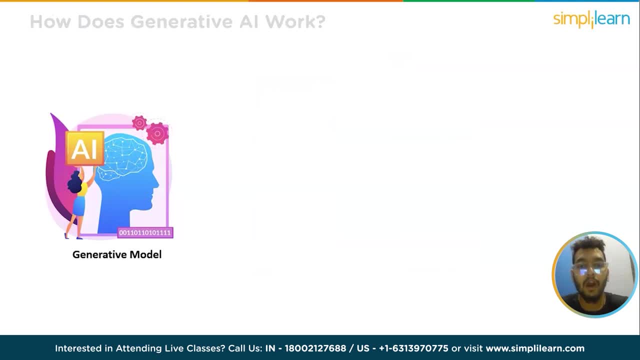 video within seconds. Now moving forward, let's see how does Generative AI work. Generative AI begins a prompt which can take the form of text, image, video, design, audio, musical notes or any input that the AI system can process. Various AI algorithms that generate. 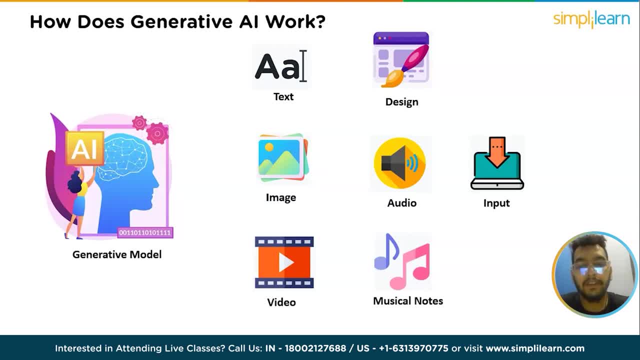 new content in response to the given prompt. This content can range from essay and problem solutions to realistic created using AI algorithms. What is Generative AI? Generative AI is a software that can generate new content created using images or audio of a person In the early stages of Generative 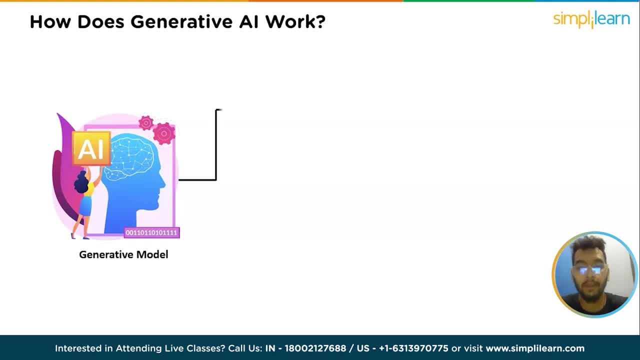 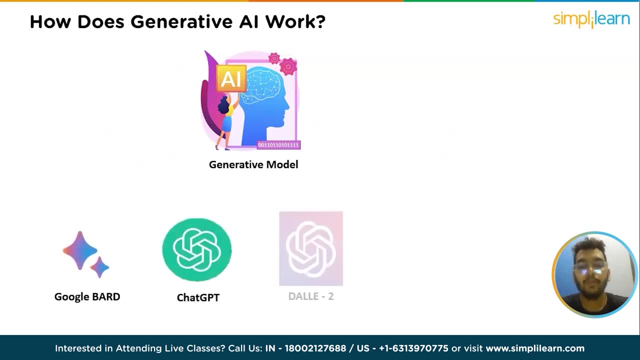 AI utilizing the technology involved submitting data through an API or a complex process. Developers need to acquaint themselves with a specialized tool and writing application using a programming language like Python. Some of the recent and fully operational Generative AIs are Googlebot, Dalai, OpenAI, ChatGPT. 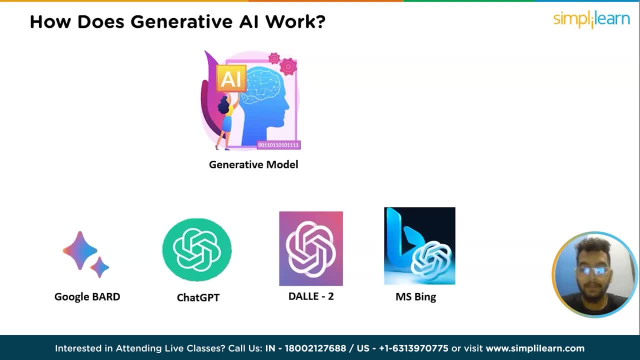 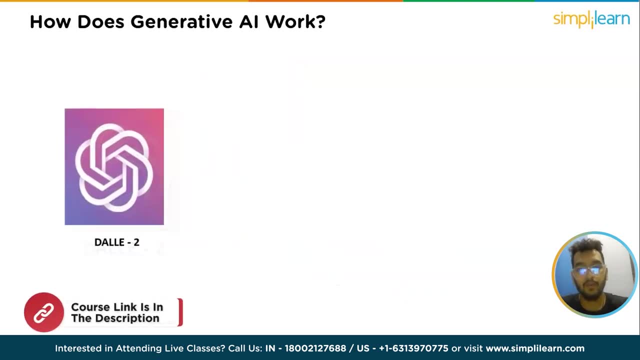 Microsoft, Bing and many more. So now let's discuss ChatGPT, Dalai and BART, which are the most popular generative AI applications. So first is Dalai 2, which was developed using OpenAI's GPT implementation in 2021. 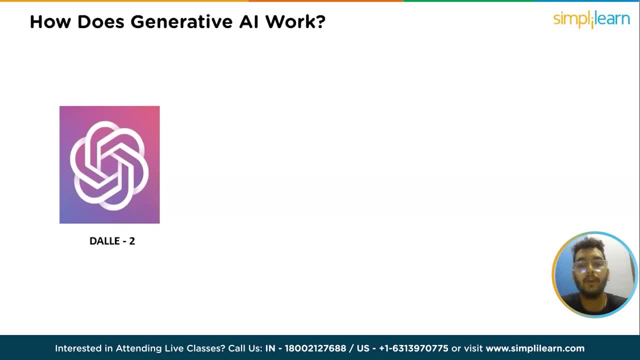 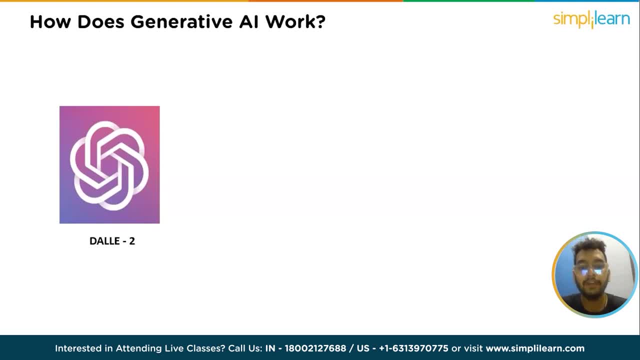 j概, And the next one is ChatGPT. In November 2022, ChatGPT, an AI-powered chatbot built on OpenAI GPT 3.5 implementation, gained immense popularity worldwide. OpenAI enabled users to interact with and fine-tune the chatbot's text response through a chat interface with. 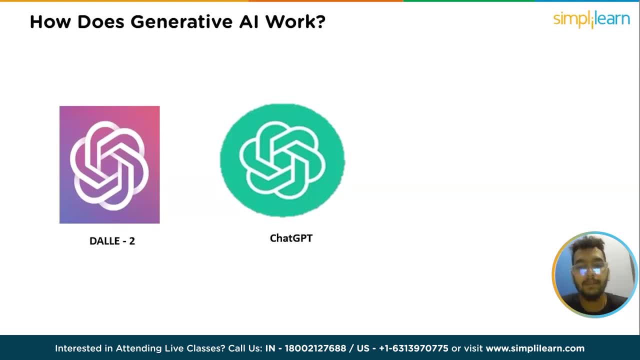 interactive feedback: Ubuntuimportance Zero. chsongcom- eastern statements accessible via an API. ChatGPT brought a more interactive experience. On March 14, 2023, OpenAI released GPT-4.. ChatGPT integrates the conversational history with the user, making a genuine dialogue. 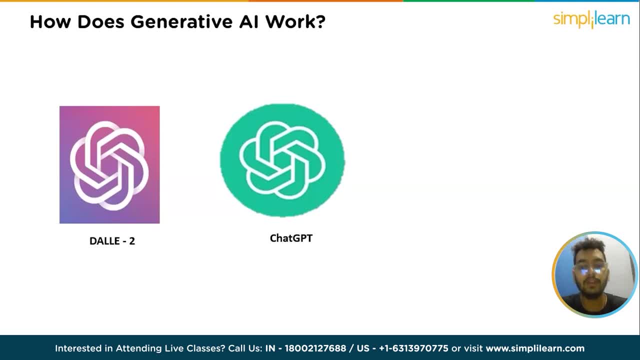 Microsoft, impressed by the success of the new ChatGPT interface, announced a substantial investment in OpenAI and integrated a version of GPT into its Bing search engine. And the next one is BARD Google. BARD Google was also an earlier fortuner in advancing transformer AI techniques for language processing. 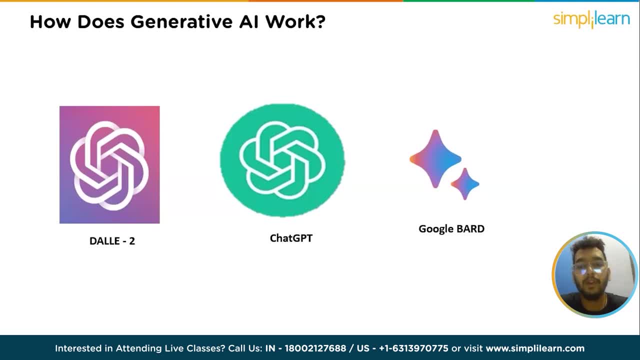 protein analysis and other content types. It made some of these models open source for researchers, but were not made available through a public interface. In response to Microsoft's integration of GPT into Bing, Google hurriedly launched a public-facing chatbot named Google BARD. 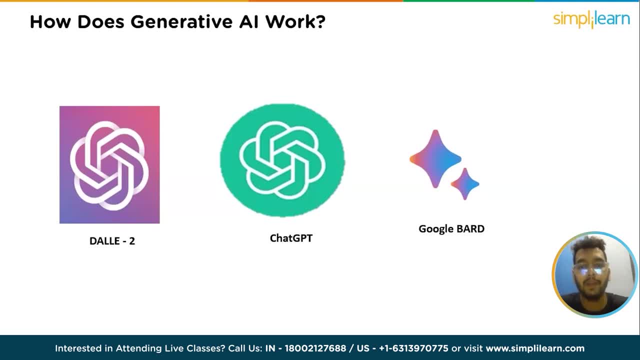 BARD's debut was met by an error, when the language model incorrectly claimed that the Web Telescope was the first to discover a planet in a foreign source. As a consequence, Google's stock price suffered a significant decline. Meanwhile, Microsoft's implementation of ChatGPT and the GPT-powered system also faced criticism. 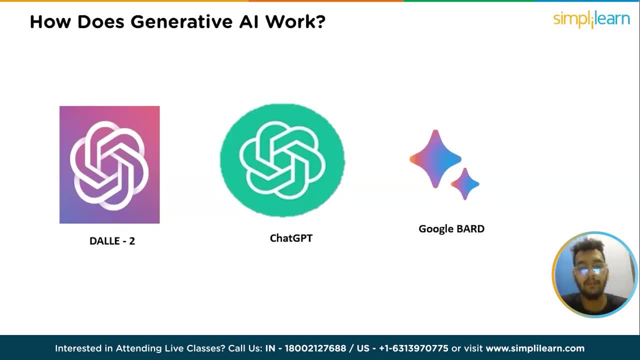 for producing inaccurate results and displaying erratic behavior in their early editions. So, moving forward, let's see what are the use cases of Generative AI. Generative AI has broad applicability and can be employed across a wide range of use cases to generate diverse forms of content. Recent advancements like GPT-4, BARD and BARD can be used to generate diverse forms of content. Recent advancements like GPT-4 and BARD can be used to generate diverse forms of content. Recent advancements like GPT-4 can be used to generate diverse forms of content. 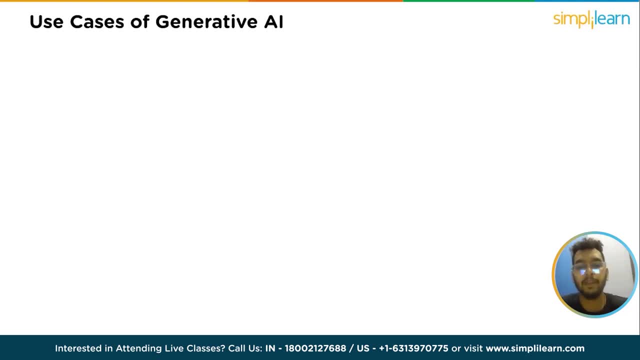 какихiding For 2 users: Q2.. Language Dubbing: Enhancement In the realm of movies and educational content. Generative AI can contribute to improving dubbing in different languages, ensuring accuracy during� champagne and high quality translation. and the third one is content writing. generative ai can assist in. 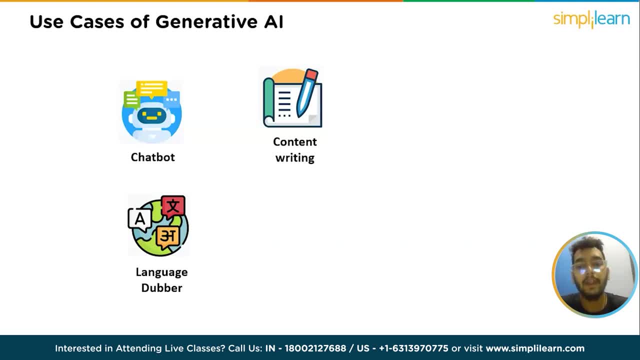 writing email response, dating profiles, resumes and term papers, offering valuable support and generating customized content tailored to specific requirement. and the fourth one is art generation. leveraging generative ai, artists can create photo realistic artwork in various styles, enabling the exploration of new artistic expression and enhancing creativity. the fifth one is product. 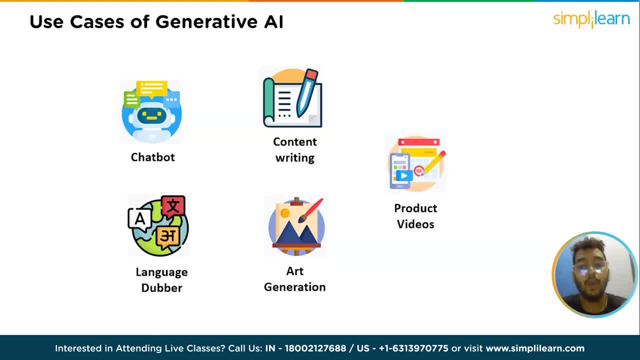 demonstration videos. generative ai can enhance to enhance product demonstration video, making them more engaging, visually appealing and effective in showcasing product features and benefits. so generative ai versatility allows it to employ it in many other applications, making it a valuable tool for content creation, enhancing user experience across diverse domains. so after seeing use case, 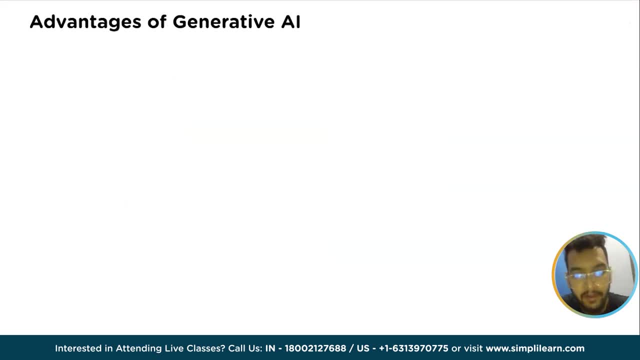 of generative ai. let's see what are the benefits of generative ai. so generative ai offers extensive application across various business domains and it is a very good tool for creating content writing and simplifying the interpretation and comprehension of existing content, while also enabling the automated creation of a new content. developers are actively exploring ways to leverage. 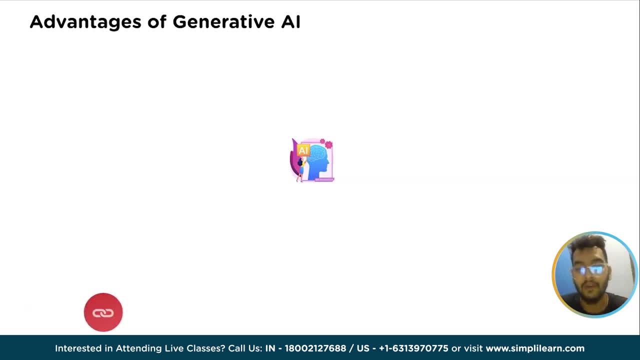 generative ai in order to enhance the optimized existing workflows and even to reshape workflows entirely to harness the potential of technology. fully implementing generative ai can bring numerous benefits, including automatic content creation. generative ai can automate the manual process of writing content, saving time and effort by generating content, creating content, writing. 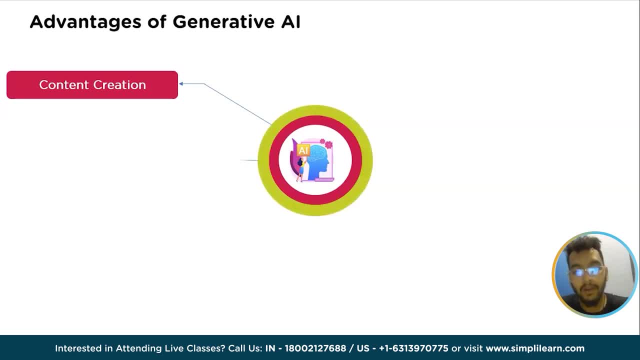 text or other form of content. the next one is efficient email response. responding to emails can be made more efficient with generative air, reducing the effort required and improving response time. and the third one is enhanced technical support. generative ai can improve responses to specific technical queries, providing accurate and helpful information to users or 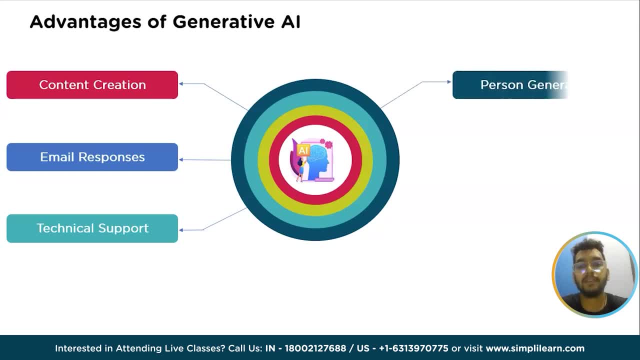 customers. and the fourth one is realistic person generation. by leveraging generative ai, it becomes possible to create realistic representation of people, enabling applications like virtual characters or avatars. and the fifth one is coherent information summarization. generative ai can summarize complex information into a coherent narrative, distilling key points and making it. 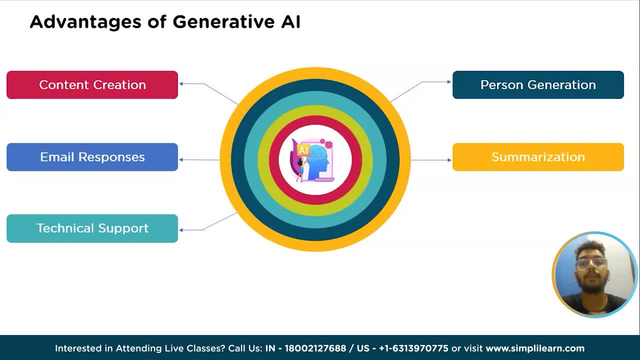 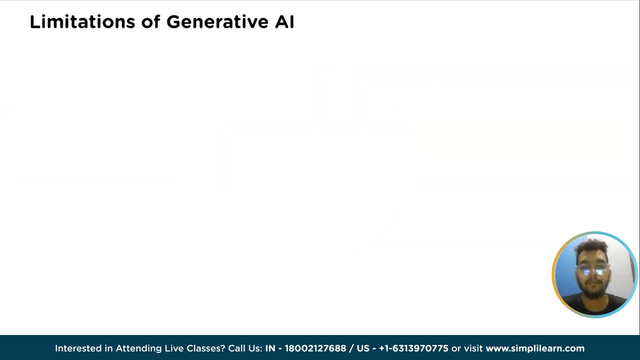 easier to understand and communicate complex concept. the implementation of generative ai offers a range of potential benefits: streamingly process and enhancing content creation in various areas of the world. so after seeing advantages of generative ai, let's move forward and see what are the limitations of generative air. early implementation of generative ai serve as vivid examples highlighting 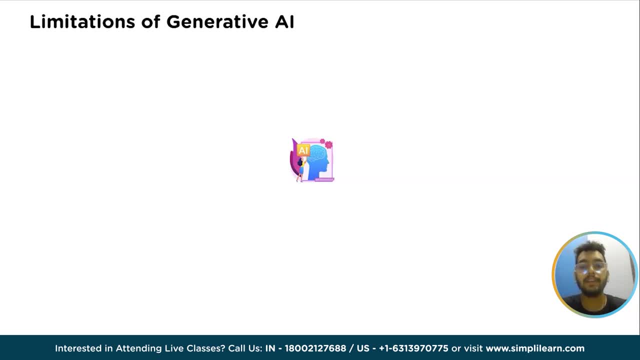 the numerous limitations associated with this technology. several challenges arise from the specific approaches employed to implement various use cases. for instance, while a summary of a complex topic may more reader friendly than explanation incorporating multiple supporting sources, the ease of readability comes at the expense of transparent information. so the first one is when implementing or utilizing a generative ai application. 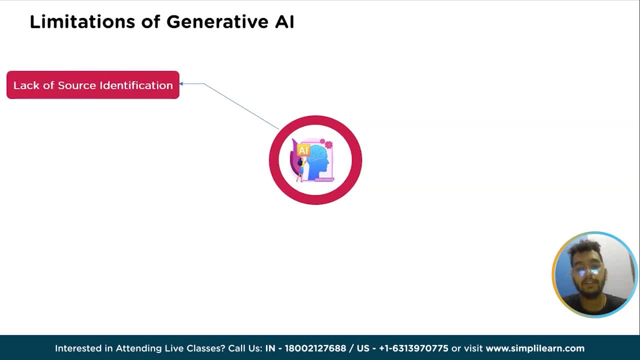 it is important to consider the following limitation. i repeat: the first one is lack of source identification. generative ai does not always provide clear identification of content source, making it difficult to trace and verify origin of the information. the second one is assessment of bias. assessing the bias of original sources used, generative ai can be challenging as it may be. 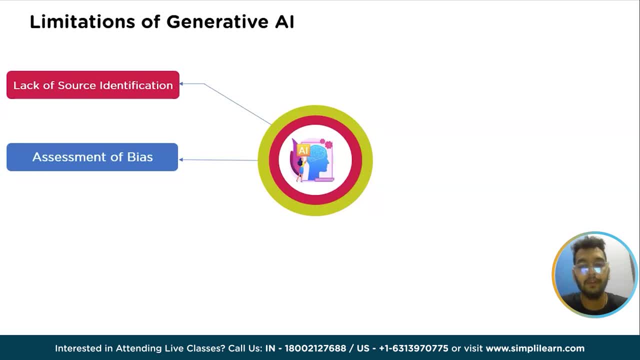 difficult to determine the underlying perspective or agendas of the data utilized in the training process. the third one is difficulty in identifying inaccurate information. generative ai can generate realistic content, making identifying inaccuracy or falsehoods within the generated output harder. and the fourth one is adaptability to a new circumstances, understanding how to fine-tune. 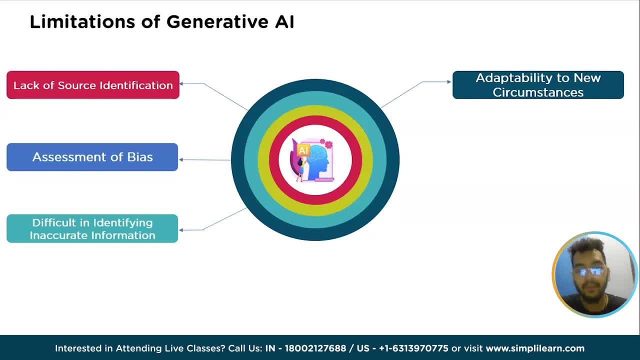 generative ai for a new circumstances or specific context can be complex, requiring consideration and expertise to achieve desired result. and the fifth one is glossing over bias, prejudice and hatred. generative ai results may amplify or perpetuate biases, prejudices or hateful content present in the training data, requiring vigilant scrutiny to prevent such.